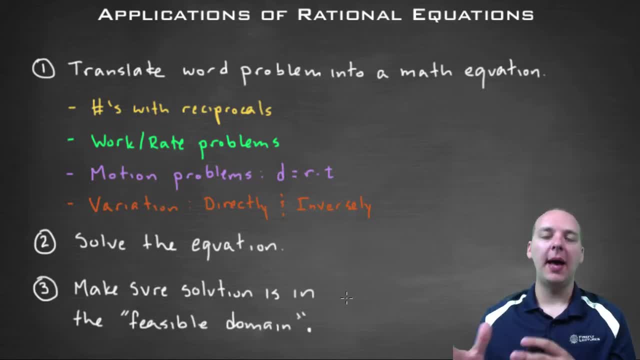 to try to translate it into a math equation so that you can solve it. For a lot of students, this is the most difficult part and, like I said, we're not going to go through the specifics in this video. We're just going to briefly identify a few different types of exercises. 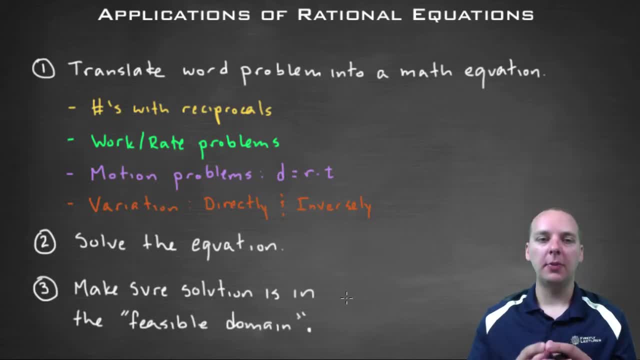 that you might see. So yeah, these are going to be real life problems. They might be work rate problems, where you know Sam can cut somebody's lawn in an hour and a half, but Susie can do it in an hour and a half. So you're going to try to translate it into a math equation. So that you can solve it. For a lot of students, this is the most difficult part and we're not, like I said, we're not going to go through the specifics in this video. we're just going to try to translate it into a math equation. It might be work rate problems, where they 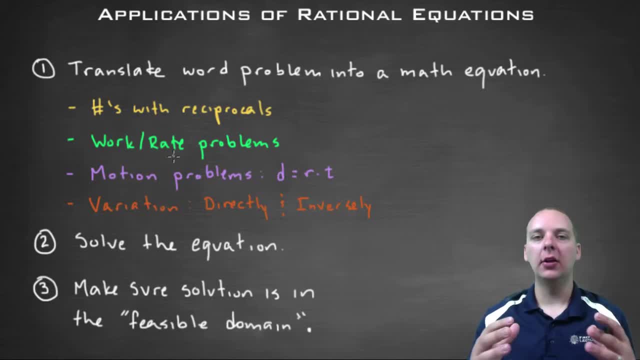 can't cut somebody's lawn in 45 minutes, so how fast can they cut the lawn? working together, That type of thing? That's a work problem. There's a way you can translate that into a math equation, but not just any math equation. it'll turn out to be a rational equation, which. 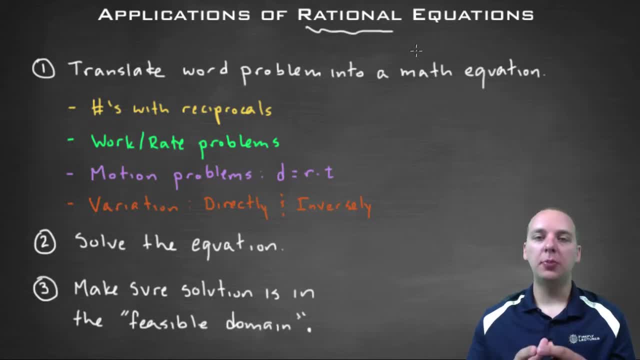 is why we're studying it right now. There's also motion problems, which is where you might have somebody kayaking up a river. that might take them two hours, but down the river downstream might only take them an hour. So how long might a river take them? an hour. So here's. 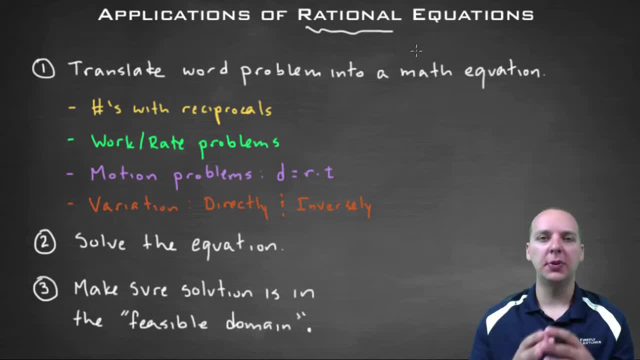 to take them to go up the river and back, and I�m being splashed with the details here, but you get the drift of what I�m talking about. We also have some more just, purely abstract examples dealing with reciprocals of numbers, because when you take a reciprocal, 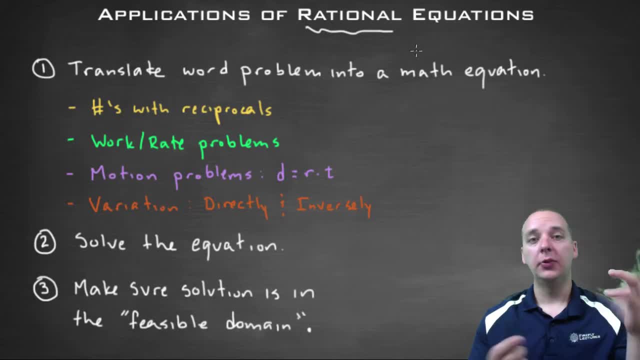 of a number, it turns it into a fraction. so if you had X, the reciprocal would be one over X. if you had that in an equation, it would make it a rational equation, of course. And then we also have some variation problems that are pretty common where you have direct 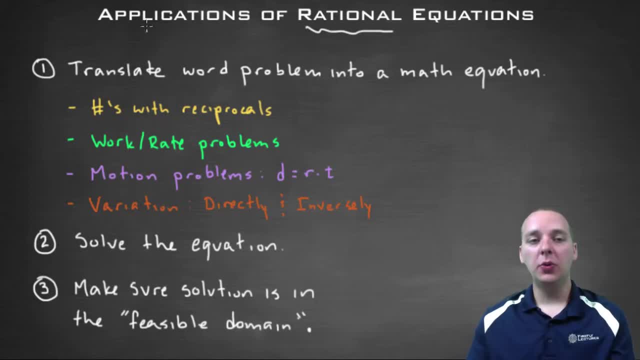 variation and inverse variation. So we�ll do examples of all of these. and again, all these word problems will turn into not just equations but rational equations. So once we set up the equation, then what do you do? Well, then you solve the equation. that should.